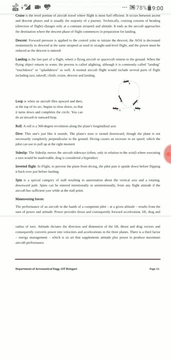 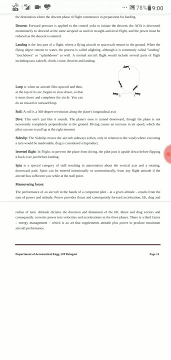 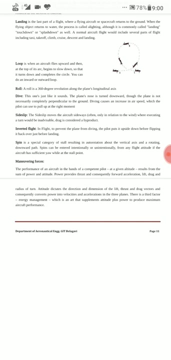 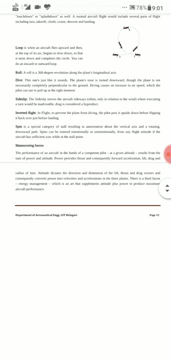 And this loop can be in inward direction as well as in outward direction, So we can call that as inward loop or outward loop. Second one is roll. Roll means when an aircraft turns 360 degree around a plane. That means if an aircraft is inverted. 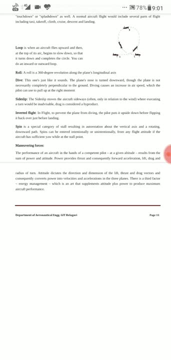 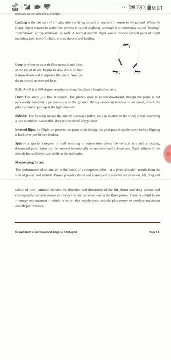 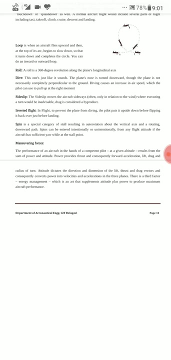 it is revolving 360 degree along the plane's longitudinal axis. That means the axis which is passing through the nose to the tail. That means it completes a roll. Next one is dive. The name itself it says that dive means diving in the air. 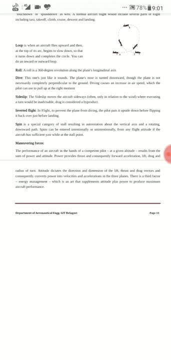 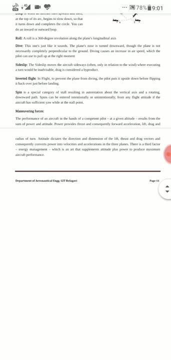 While diving, the plane's nose will be in the downward path And not necessarily it should be perpendicular to the ground. Next one is side slip. The side slip maneuver will occur when an aircraft is taking a turn in sideways, And this will create a drag. 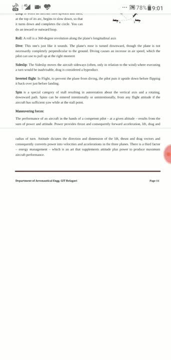 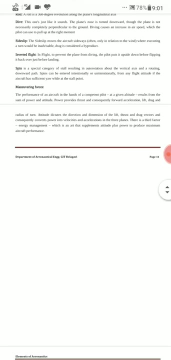 Therefore the side slip is not advisable. To overcome from side slip, pilot must operate the rudder part and keep the aircraft stable. Next one is inverted flight. If the aircraft is upside down, we can call that as inverted flight. The last one is spin. 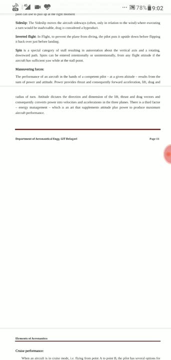 That means when an aircraft starts at a rotation about the vertical axis by rotating in the downward path, then that is called as spin, And spin can be done intentionally or unintentionally with respect to the altitude. Thank you.